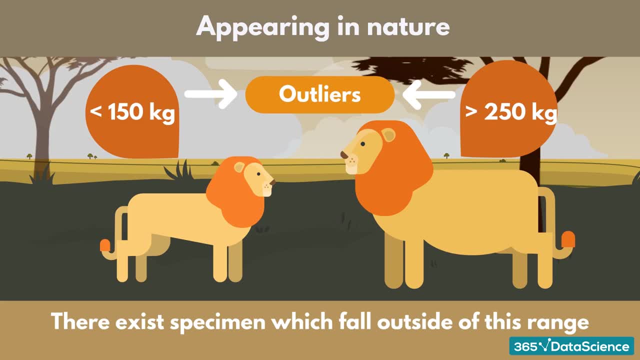 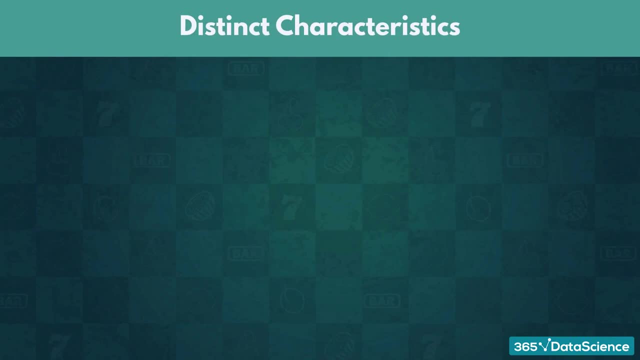 of the data they represent. Now that you know what types of events follow a normal distribution, let us examine some of its distinct characteristics. For starters, the graph of a normal distribution is bell-shaped. Therefore, the majority of the data is centered around the mean. Thus, values further away from the mean are less. 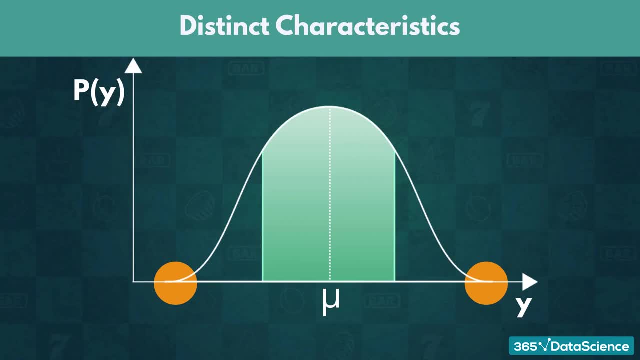 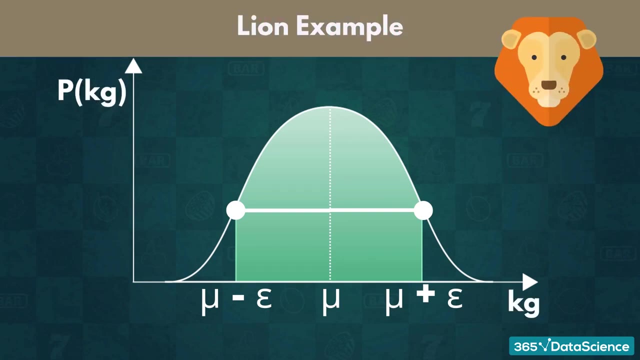 likely to occur. Furthermore, we can see that the graph is symmetric with regards to the mean. That suggests values equally far away in opposing directions would still be equally likely. Let's go back to the lion example from earlier. If the mean is 400, symmetry suggests a lion. 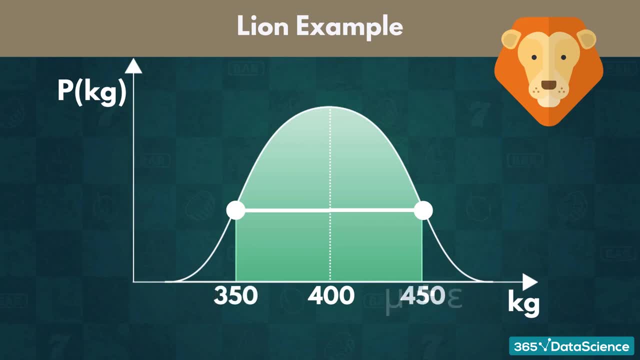 is equally likely to weigh 350 pounds and 450 pounds, since both are 50 pounds away from the mean. Alright, instead of going through the complex algebraic simplifications in this lecture, we are simply going to talk about the expected value and the variance. The expected value: 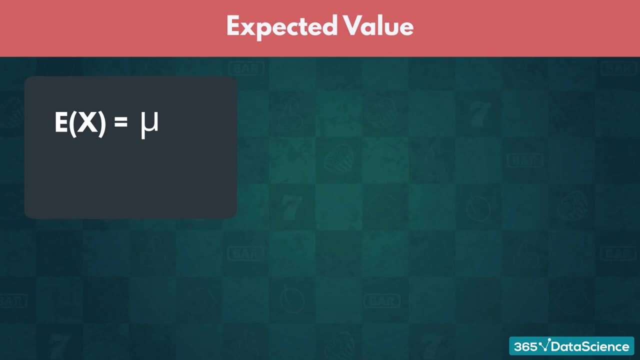 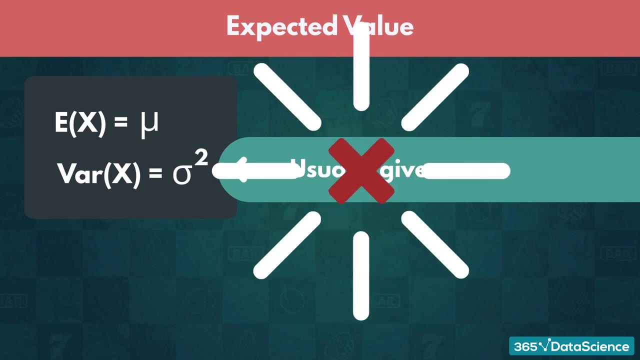 for a normal distribution equals the expected value. This means that the expected value distribution equals its mean mu, whereas its variance sigma squared is usually given when we define the distribution. However, if it isn't, we can deduce it from the expected 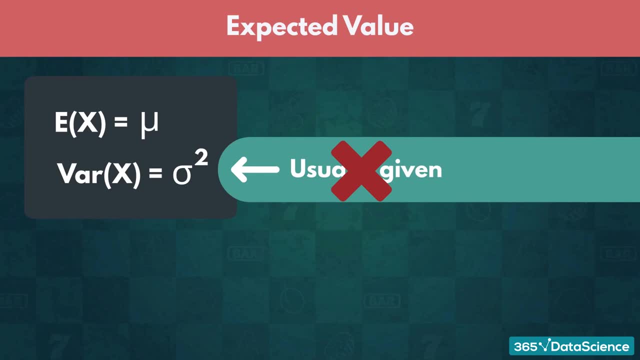 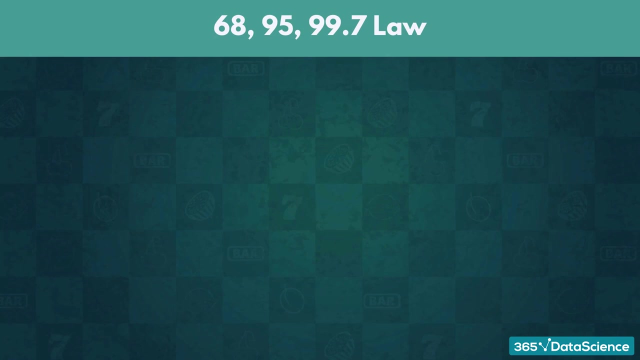 value. To do so, we must apply the formula we showed earlier. The variance of a variable is equal to the expected value of the squared variable minus the squared expected value of the variable. Good job. Another peculiarity of the normal distribution is the 68-95-99.7 law. This law suggests that 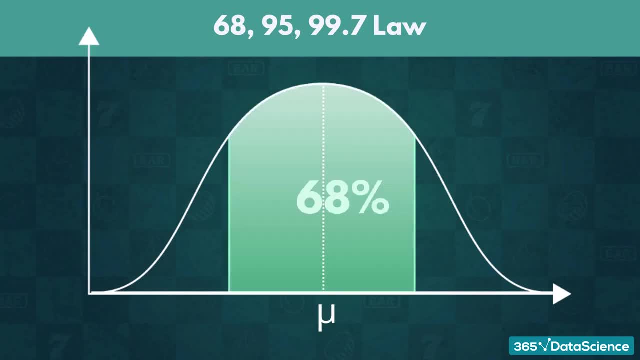 for any normally distributed event, 68% of all outcomes fall within one standard deviation away from the mean, 95% fall within two standard deviations and 99.7 within three. The last part really emphasizes the fact that outliers are extremely rare in normal. 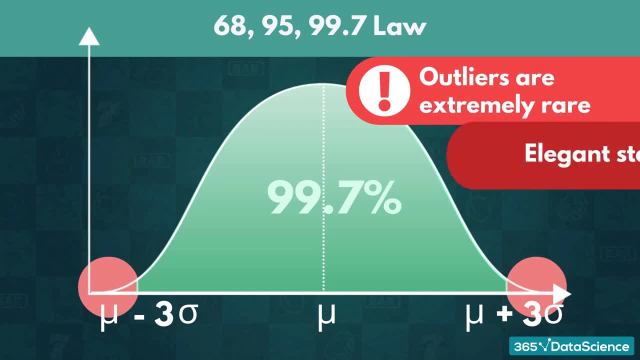 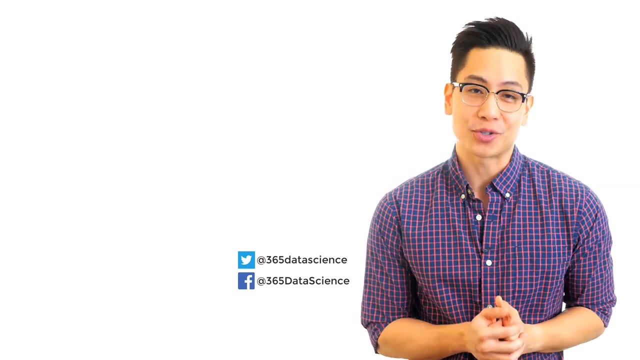 distributions. It also suggests how much we know about a dataset if we only have the information that it is normally distributed. Fantastic work everyone.